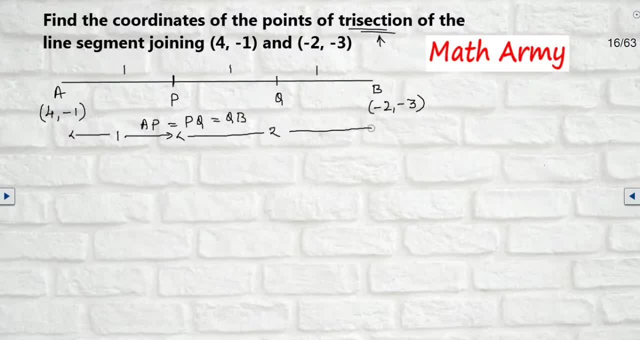 is divided by p in the ratio of 1 is to 2.. Now, from q point of u, the same line, segment a, b is divided into 2 is to 1.. From a to q is 2.. Okay, and from q to b is 1.. 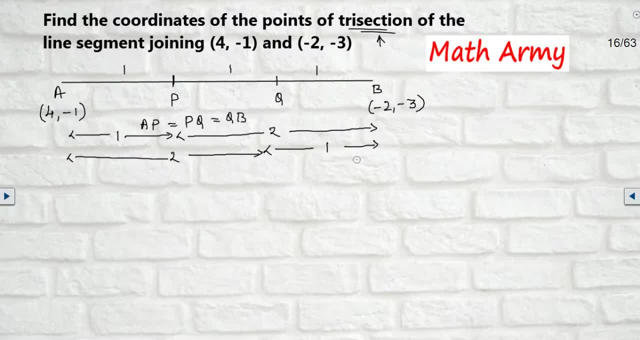 So that is how you need to understand. So here, from p point of u, the ratio of is divided in 1 is to 2.. From q point of u, it is 2 is to 1.. Now I am going to use the section. 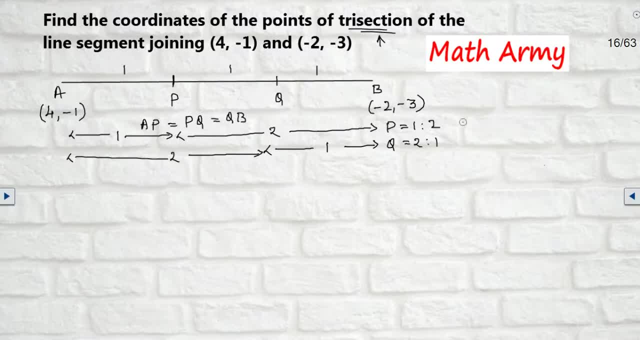 So, before getting into the section, formula for p, m1 is to m2 is 1 and 2.. Okay, and for q, m1 is to m2 is 2 is to 1.. And that is the major difference. You need to understand it. And x1, y1 and x2, y2 are the 1 and the same in both the cases. 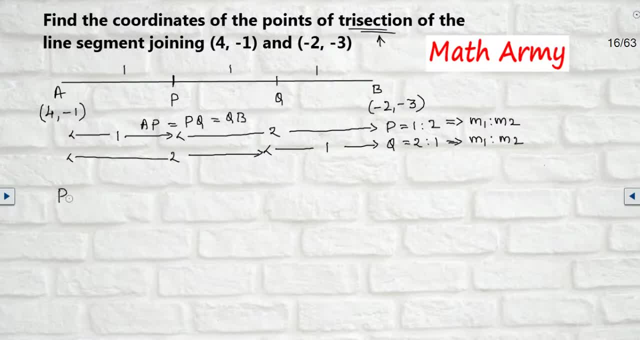 Now I am going to use the section formula for p. And what is the section formula? M1, x2 plus m2, x1 divided by m1 plus m2, comma: m1, y2 plus m2, y1 divided by m1 plus m2.. Okay, 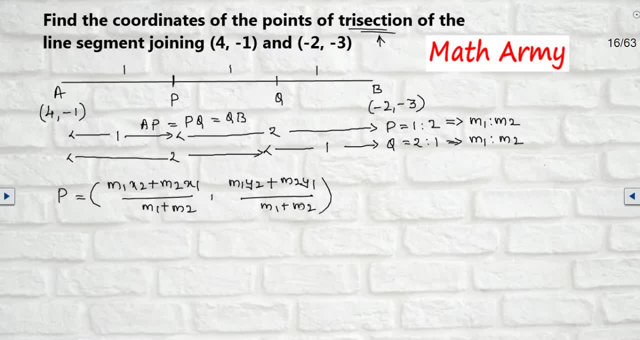 Now put all the values here. What is m1? p? it is 1.. So 1 multiplied with x2.. x2 is minus 2.. So let me write the x1, y1 and x2, y2.. 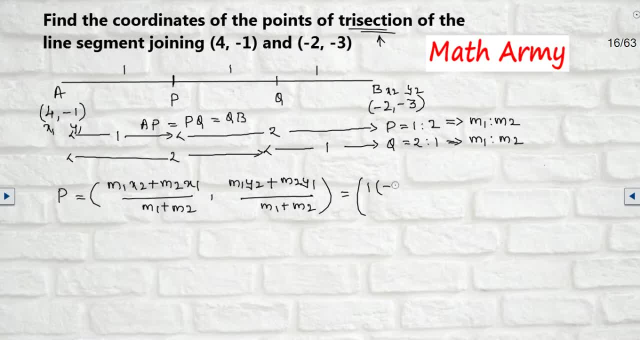 Now, 1 multiplied with minus 2 plus 2, multiplied with x1, which is 4, divided by m1 plus m2, which is 1 plus 2, again m1,. 1 multiplied with y2, which is minus 3 plus 2, multiplied with minus 1 divided by 1 plus 2.. 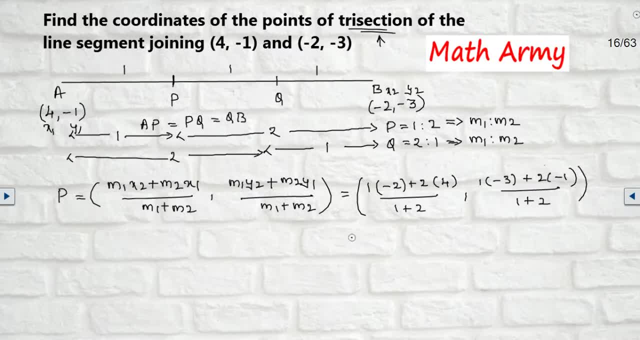 Now, on calculating, you will be getting minus 2 for 2's height. So plus 8 divided by 1 plus 2 is 3.. And here it is minus 3.. Okay, and minus 2.. I am directly writing: minus 5, guys divided by 3.. So, guys, here, minus 2 plus 8 is 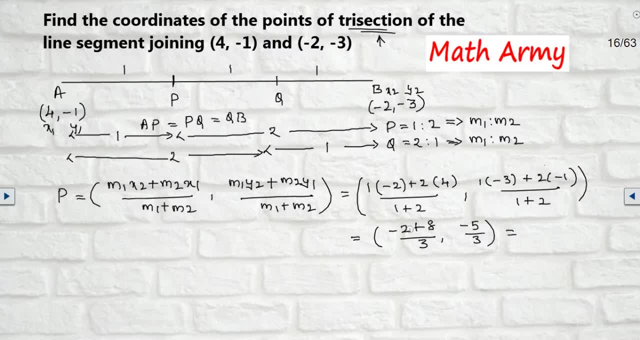 plus 6.. 6 divided by 3 is 2.. So directly I am writing 2 comma minus 5 by 3, and this is the value of section P. So write here: 2 comma minus 5 by 3.. This is one of the answer. Now let us find. 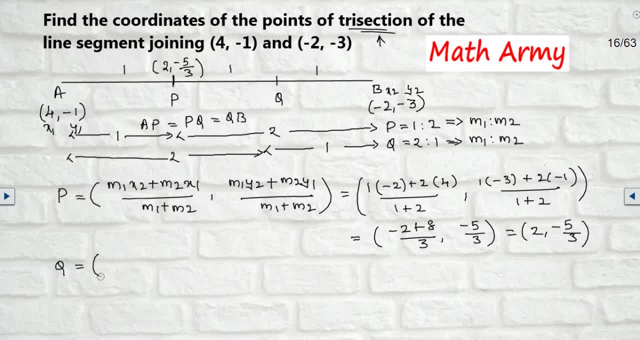 for Q. Same formula, but the ratios are: 2 is to 1, not 1 is to 2.. This one, Okay. 2 is to 1.. So this is a major difference between P and Q. X1, Y1 and X2, Y2 will be the same. Okay, Now 2 multiplied. 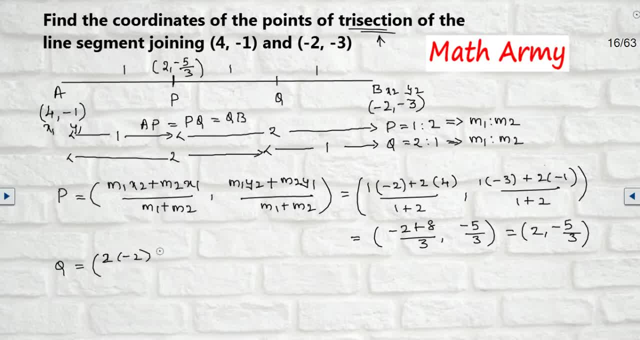 with 2.. So this is the value of section P. So write here: 2 comma minus 5 by 3.. This is one of the answers. Now write here: 2 comma minus 5 by 3 plus 1, multiplied with minus 2 plus 1 multiplied. 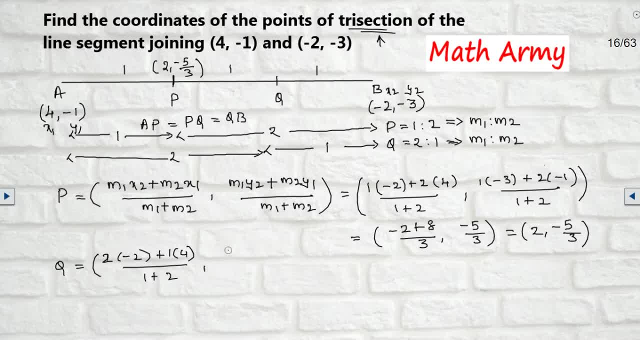 with 4 divided by 1 plus 2, comma 2 multiplied with minus 3 plus 1 multiplied with minus 1 divided by 1 plus 2.. Now, 2 multiplied with minus 2 is minus 4 plus 4 divided by 3.. This is the. 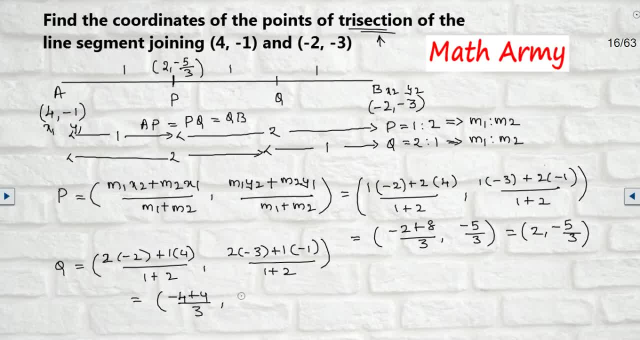 and minus 6 mean minus 1 divided by 3. now minus 4 plus 4 is 0. 0 by 3 is 0 comma minus 6 minus 1 is minus 7 by 3, so q value is 0 comma minus 7 by 3. 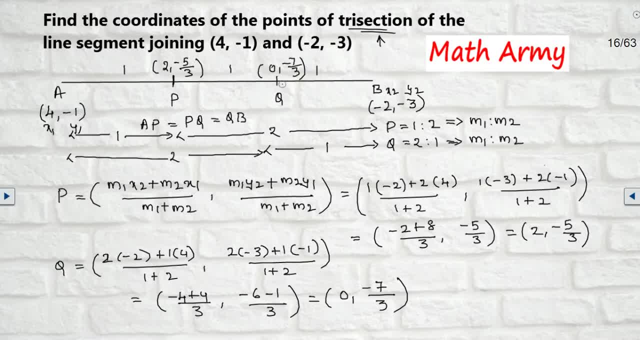 and that's it, guys. these are the p and q values. if you like my explanation, please don't forget to share and subscribe to my channel. see in the next video. bye for now.